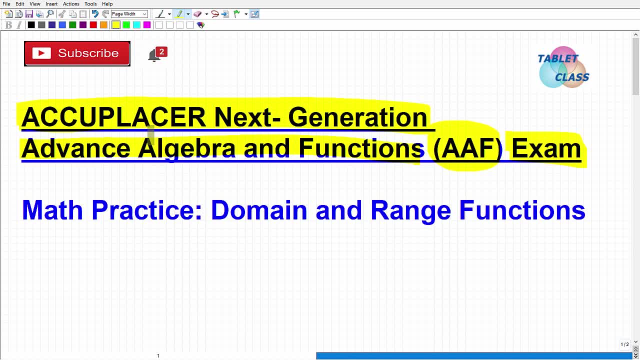 your require you to study and this, this AAF exam, this is a significant exam, okay, and there's a lot of mathematics on here and you're gonna want to put the time in and it's not enough for for someone to say: well, I took algebra and I did really good in high school. I took your algebra 2 pre. 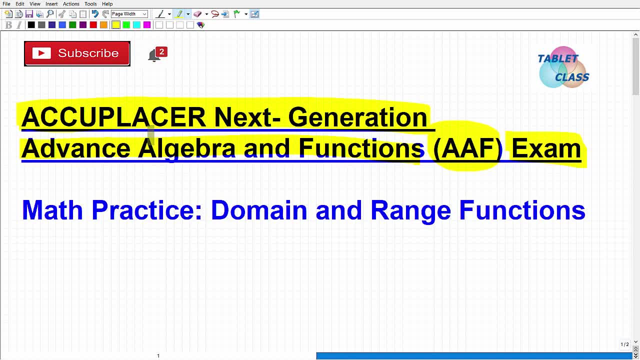 calculus and all trig. I was all really good in geometry. it doesn't make a difference. if you took the the courses and you were good in them, okay, it what? that is very important. but what's more, probably even more important, is how long you've been away from the subject. okay, how much your retention level. so you. 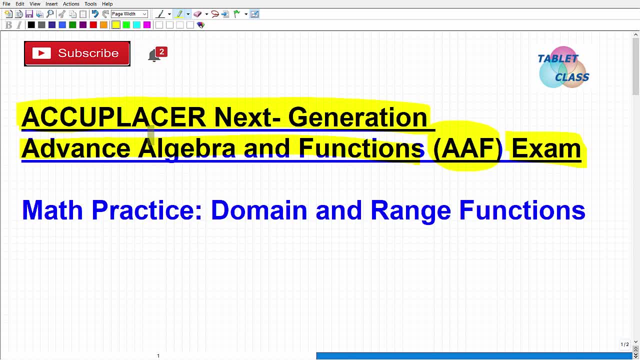 have to really get back into a state of immersion. I'm doing a lot of proms. you're familiar, nurse, re familiarizing yourself with all these concepts so you can walk into this exam with confidence. now, with that being said, if you're looking for kind of a good study program and you like my teaching style, I offer a. 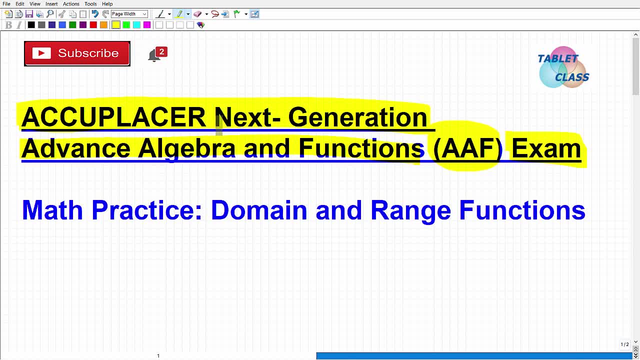 specific course for the ACCUPLACER next-gen AAF exam. I'll leave the link in the description. this is my test prep course that I designed very comprehensive, so if you're looking for something specific, you can check that out, and there's other things out there that are available to you as well. so with 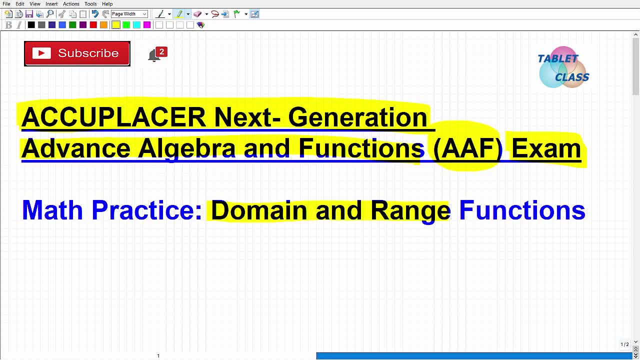 that being said, let's talk about one small but extremely important topic that you're gonna have to know for this exam, and that's domain and range of functions. now, this is a huge topic and I'm not. I'm gonna just kind of scratch it a little. 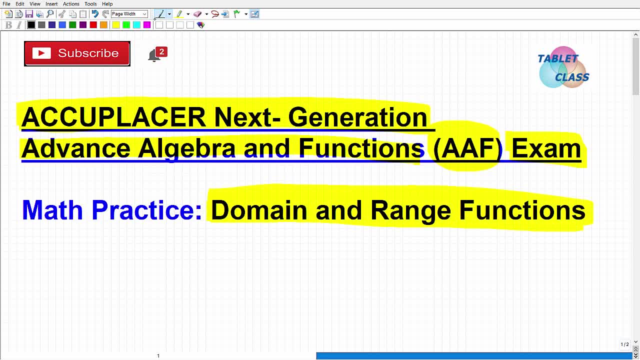 bit. I'm gonna just be talking in very broad terms but highlighting some things that that you can kind of gauge off of what I'm talking about: whether you know. whether you know, if you understand what I'm saying, then that's pretty good, but if you're like boy, I don't really understand what he's saying. 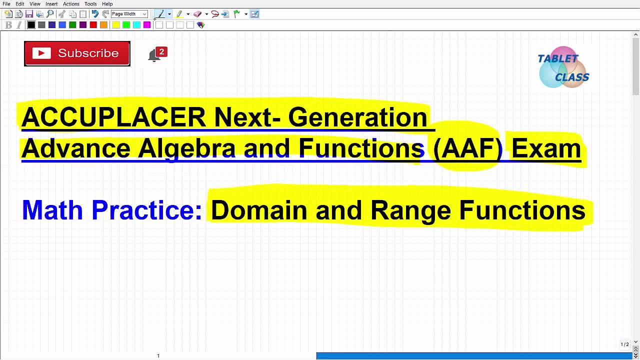 then that's a big red flag that you need to go back and and do some serious studying. but even if you understand what I'm talking about, that's still not like an indicator that, oh yeah, you're good to go for the test, right? so again, lots of. 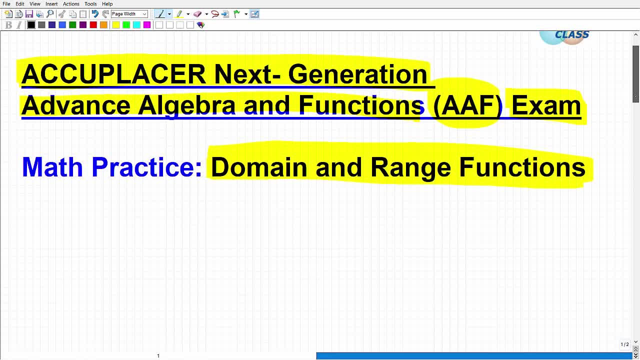 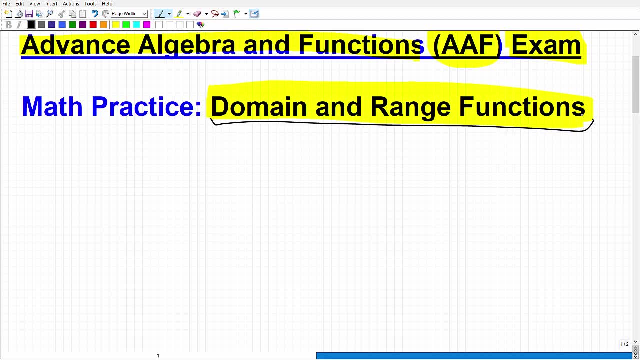 lots of mathematics. on this particular example, let's talk about domain and range and make the most of it for this video. so, domain, a range of functions. well, in mathematics, okay, we have something called relations, relations- all right, big topic- and relations are essentially XY points on the XY plane. okay, I'm speaking very, very broadly here, okay, but 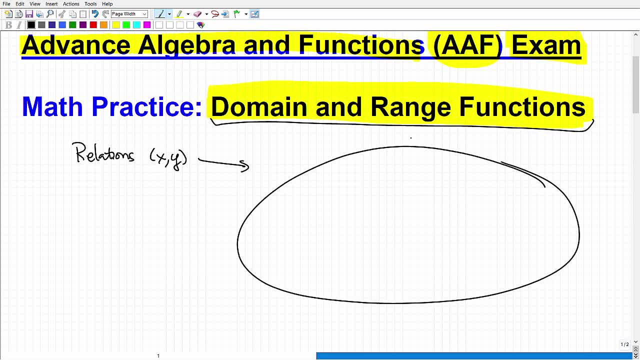 that's basically what they are. and so in this broad world of mathematical relations, okay, a subset of relations is something called functions. all right, huge, super important topic in mathematics. okay, so functions are a type of relations, okay, and there's Test to determine if something is a function, right. so one thing would be like the vertical line test, um. 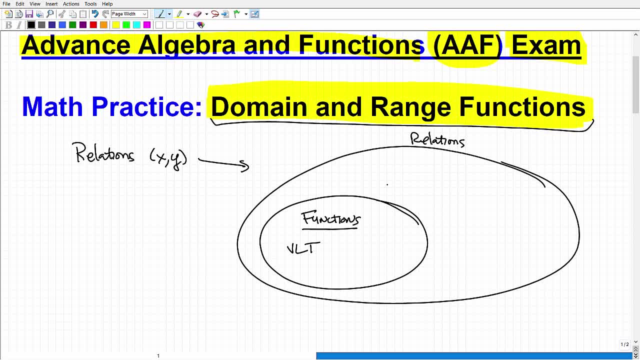 and then there's other ways to kind of look at to determine if something is in fact a function. now, if something is a function, then uh, there's all different type of things we can uh, different ways we can express it, different things we can think about it, etc. and one of the most important things is domain and range. so 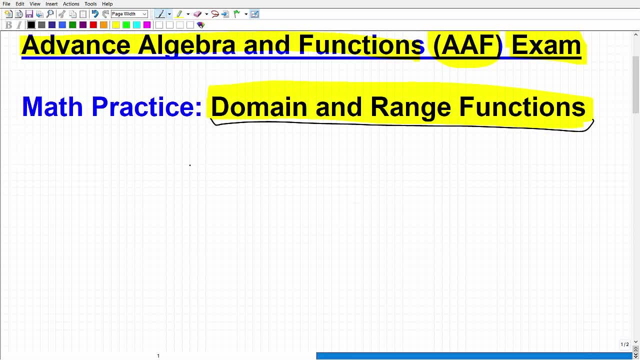 now let's kind of erase this here. so let's look at a real basic function here. okay, so this is a function, right? so we have f of x equals 2x plus 1, and i'm skipping over all kinds of stuff right now, uh, so in no way this is is this kind of like a formal lesson on functions, and 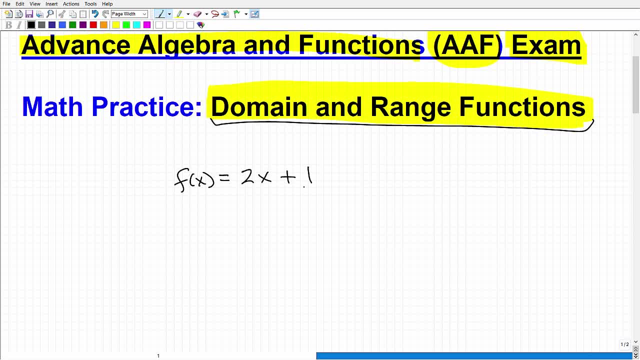 everything else. but you know again, that's not the purpose of this video. this video is just to kind of get you, you know, thinking about this and seeing where you're at all right. so here is a function we were uh. we say: this is f of x equals 2x plus 1, and i'm skipping over all kinds of stuff right now. 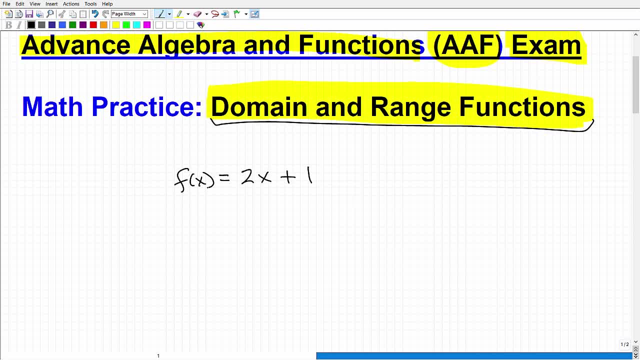 f of x equals 2x plus 1. now the way this works is: we can evaluate this function. right, this is a rule, okay, so what it means is this: x here. if i put in a number like, let's say here, like two, let's use a. 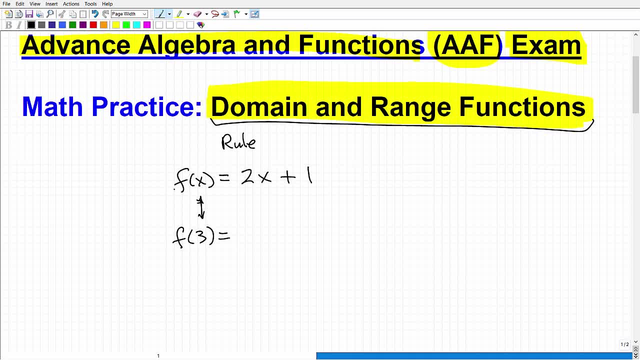 different number, let's say three. i want, i would want to evaluate the function for three. okay, f of three. i'm trying to find out what is the value of f of three. well, the rule says this: this 2x is said to be f of x equals 2x plus 1, and i'm skipping over all kinds of stuff right now. 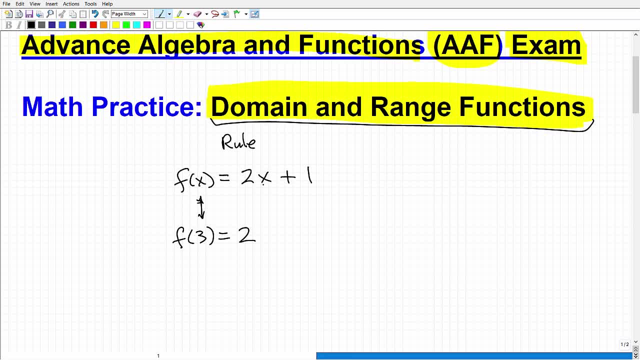 f of x equals 2x plus 1 and it says: whatever number you put in here, just replace all the x's you see over here. so this x is this is 2 times x. so it's going to be 2 times 3 plus 1. so f of 3. 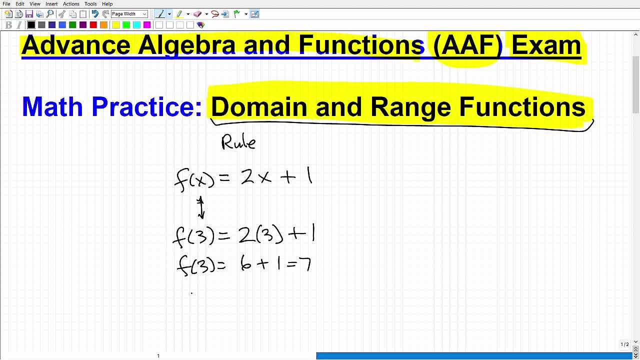 will be what? 2 times 3 is 6 plus 1 or 7, right? so f of 3 equals 7, okay, so this is a basic function here and let's go ahead and write it over here. so it's a rule, okay. now, what i want you to think about this rule is this: this x represents the. 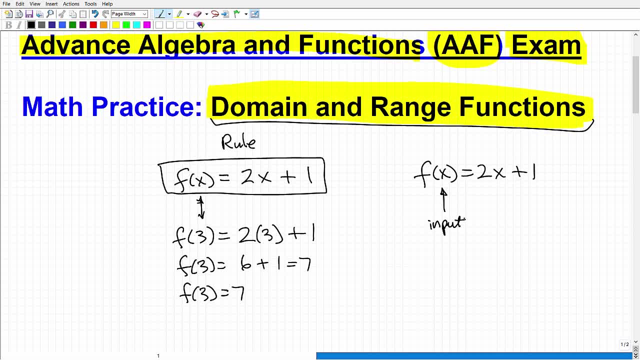 input value: the input value. okay, so i'm going to put something into the function. in this case it was three, and then when i finished up doing whatever i had to do, i got an output value, output right and that was seven right. so in this example, i, my input was three and my output was. 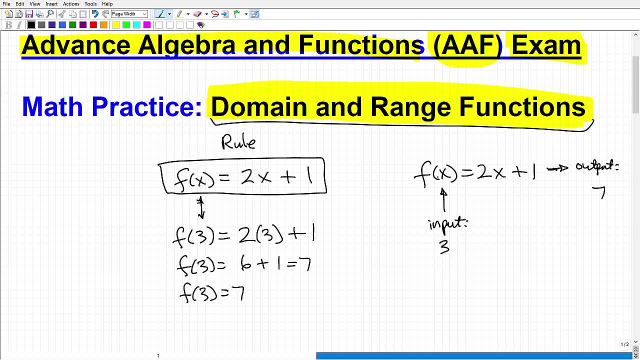 seven, okay, so i put something into the function rule and then i kind of spit out this number. in this case it was seven. so, more formally, when you're dealing with the function, your input values, the numbers, the values you put in, are called the domain. okay, and then on a particular function, all. 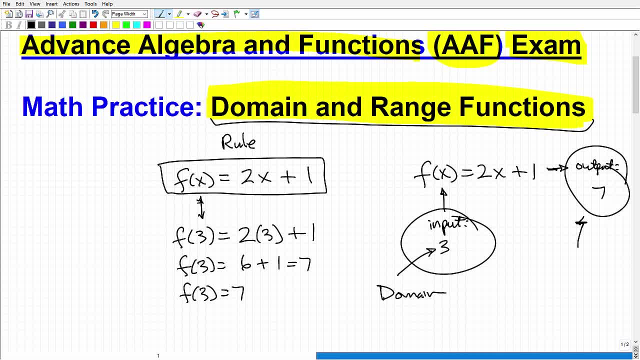 the output values that you can get is called the range. all right, so if you're with me so far and you're like, yeah, i'm going to put in the input value and then i'm going to put in the output value- yeah, i kind of remember that i get that- then fantastic, okay. so this is where i want to kind. 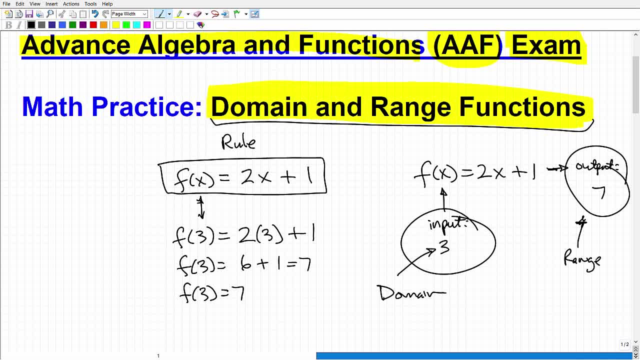 of take this uh video here and talk, you know, just a little bit more advanced. okay, so in domain and range there's, specifically with domain, there are, there can't be restrictions and they, uh, there certainly will be restrictions on some functions. so, let's, let's talk about actually, let's, let's. 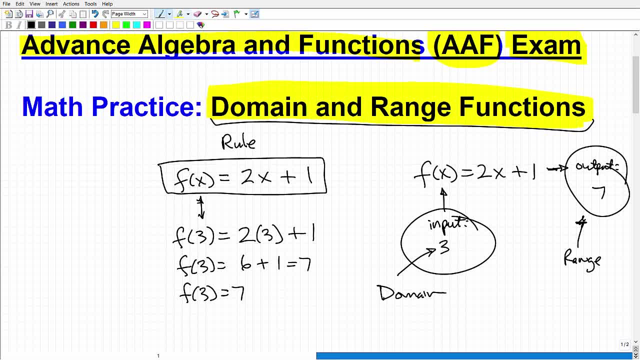 stick with this problem here for a second. so if i asked you what is the domain, what is the domain of this function, you should be able to tell me what the domain is. okay, so the domain is not three. okay, i could put in any number here. i could put in. 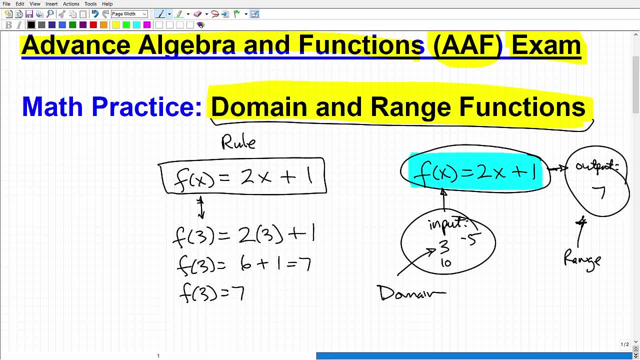 10. i could put in negative five, right. i could put in zero, i could put any value, and when i plug it in and i replace this x with any one of these values, i'll get some sort of number right. so in this particular function the domain is the set of all values i can plug into the function. all right, that's the. 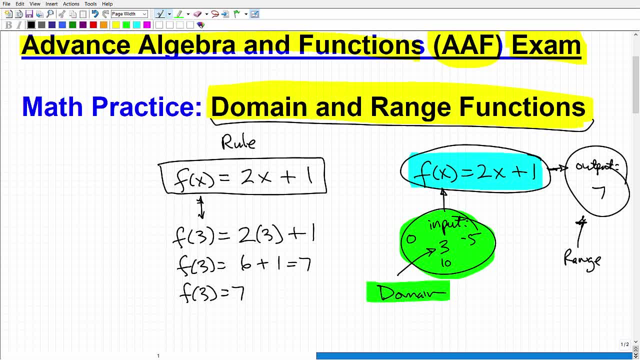 question when we're talking about them- and let me just back up here for the purposes of the af exam- you're going to be we'll be dealing with complex numbers, but we're dealing with uh, domain and range function questions. you're probably generally going to be, uh, restricted to the real number set. 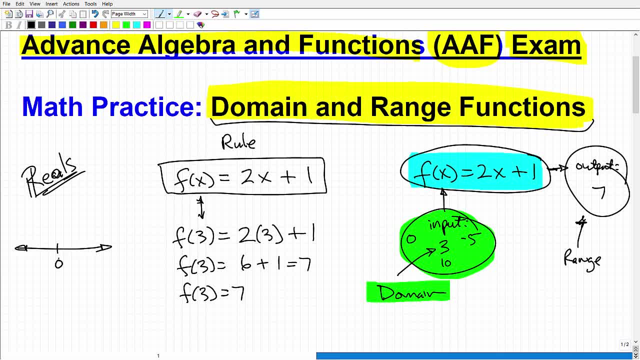 okay, the real number set. okay, the real number set. but we're gonna um figuring out what actually is the real number line. so here's a number line, right, zero in the middle, all your positive numbers over here, all your negative numbers over here. this is the real number system. okay, if you're already kind of lost. 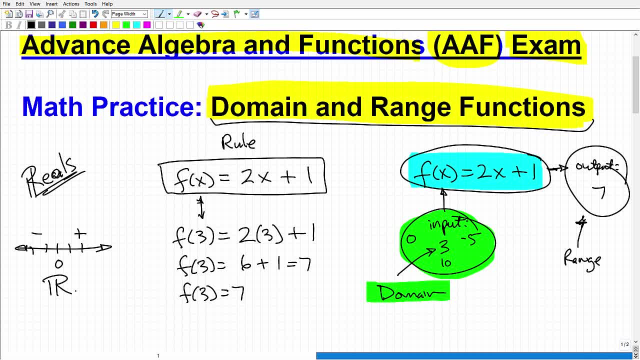 what i'm talking about. that's a big like alarm bells going off. today you got some studying to do. okay, again, this test is comparable to what you would want to be, you know, at a high level for like the sat or eight or act. okay, it's advanced. that's just algebra. this is the these, this topic. 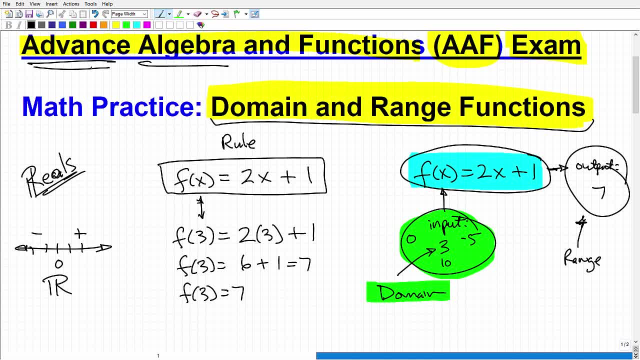 advanced algebra. okay, all right, so let's continue to press forward here. so the domain, more formally, is the set of all input values that you can you can plug into the function. so in this case there is no restriction. i can plug in any number along the real nine, the real number line, and it'd be. 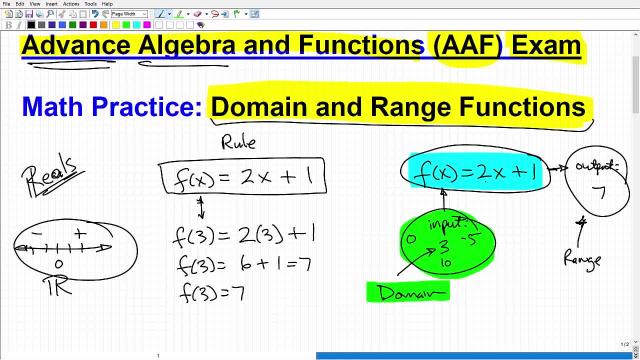 okay, right, i can plug in a negative value, i'll get a number out. i can plug in zero, right, two times zero, zero plus one. so my answer would just be one: there's, everything's fine. so my domain in this case is the set of all real numbers, and there's a lot of ways we can express that. 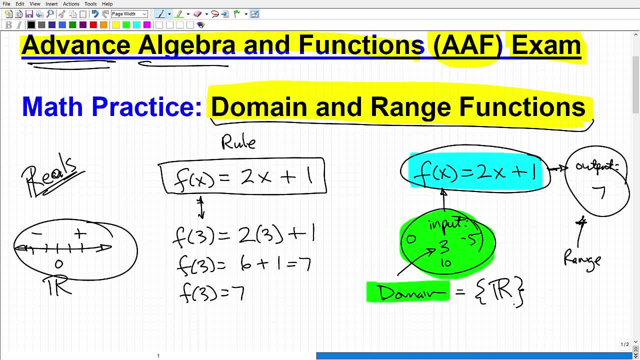 this is one way that we can do it, but that's basically it. so i can plug in any real number along the real number line into this function. it's not going to hurt it. i'll always get a number out and my range will be all real numbers as well. okay. 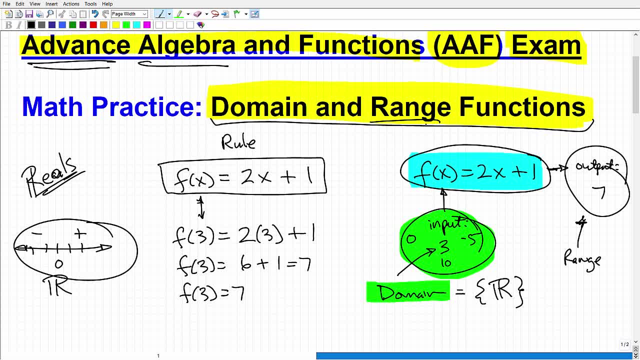 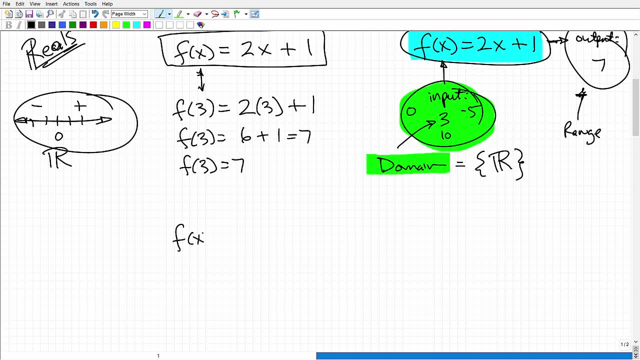 so, so pretty straightforward stuff. hopefully you're you're, you're with me. but let's move this forward a bit. okay, i want to talk about functions, uh, and where we can get in trouble. so it's basically, let's do something like this: i'm going to write two functions here. 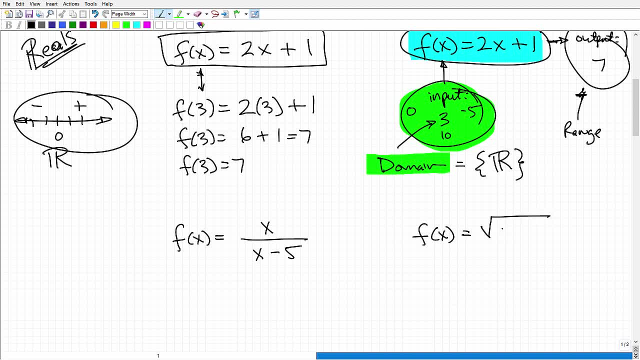 and i'll tell you what i'm doing in a second. okay, so now let's just discuss what the domain could be for these particular function. okay, these functions here. all right, so here we have a function, we have a rational function. okay, so i can plug in- here's my input values, right? so if i'm trying to find, let's say, f of one, let me give. 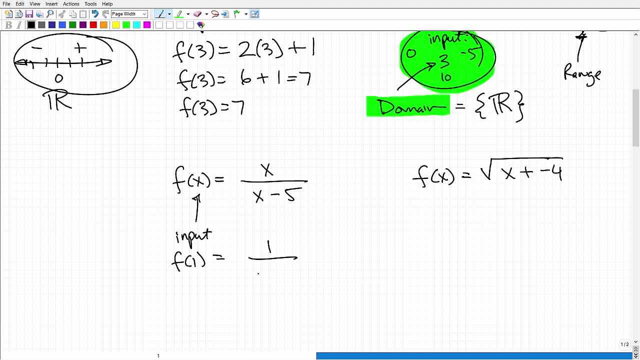 myself some more time here. let's see if i can find f of one. let me give myself some more time here. let's room, it would be what It would be? 1 over 1 minus 5, right, I'm going to replace these. 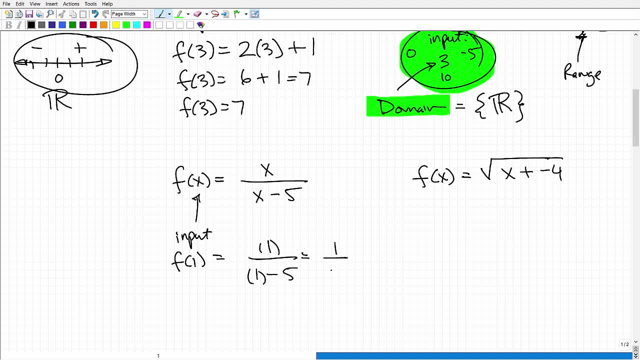 x's with 1, and I'm going to get 1 over negative 4,. okay, And that would be good to go. That's my answer. So f of 1, f of 1 is negative. 1 fourth: No problem, Let's take a look at this. 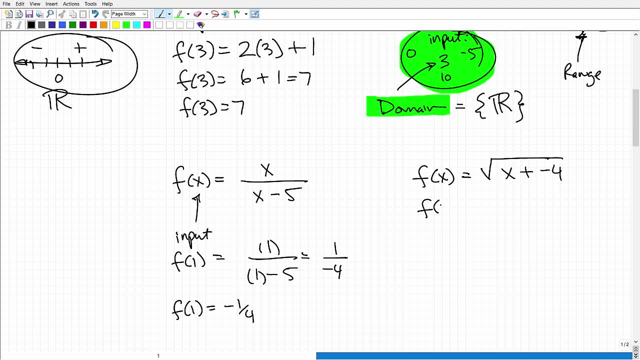 function over here. Let's say I was trying to find f of 2.. Okay, no, let's not do that, Let's do f of 10.. That would be what I would replace this x here with 10, so 10 plus negative. 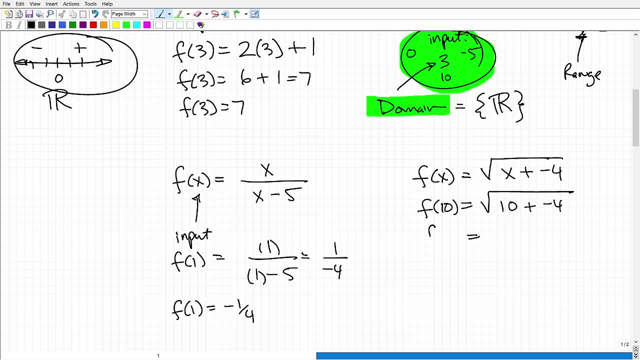 4 is going to be 6, so f of 10 will be the square root of 6.. Okay, so still, we're evaluating these functions. No problem, So far, everything looks pretty good. okay, Let's go back to. 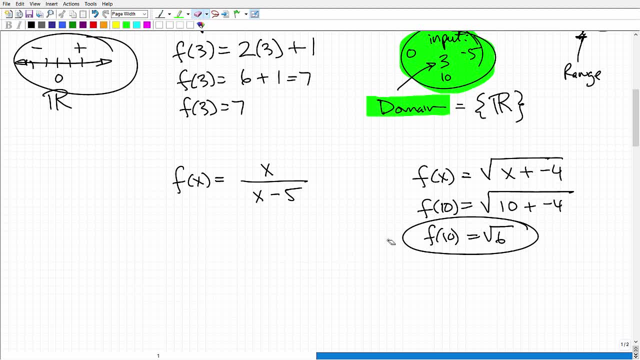 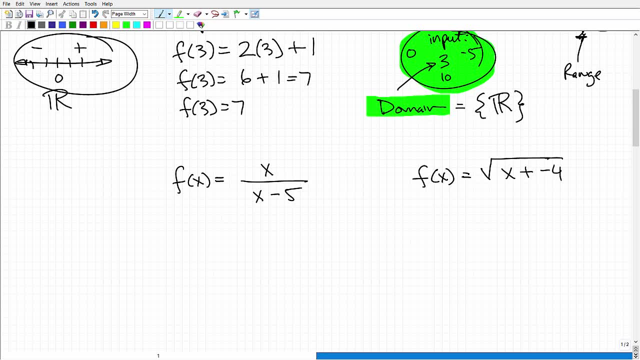 same. So I have two functions and they're the same. So I have two functions and they seem to be okay. But if I ask you, what is the domain on these functions? well, these two examples I picked out here, we have restrictions. okay, It's not going to be so nice and easy. 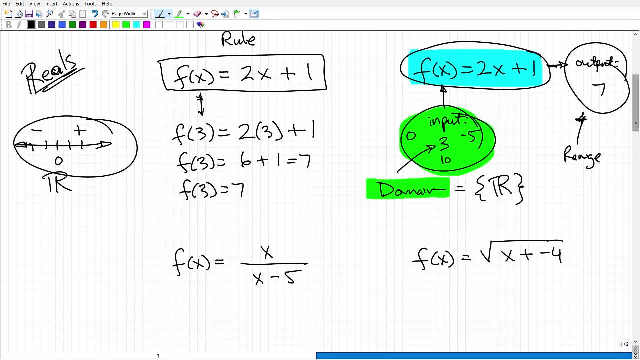 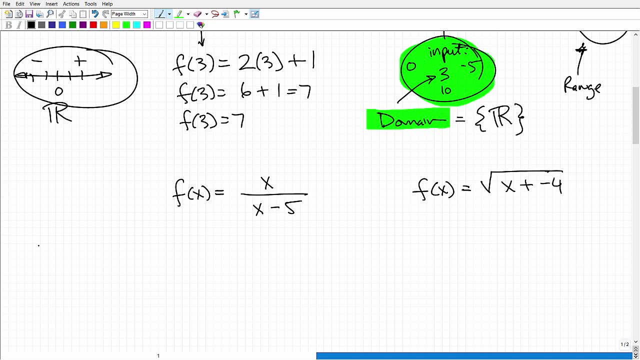 as our first function here, where the domain is all real numbers. So what am I talking about? Well, there's two things you need to know about when talking about domain and functions. The first is this: You can never in a function, we can never- end up with zero. 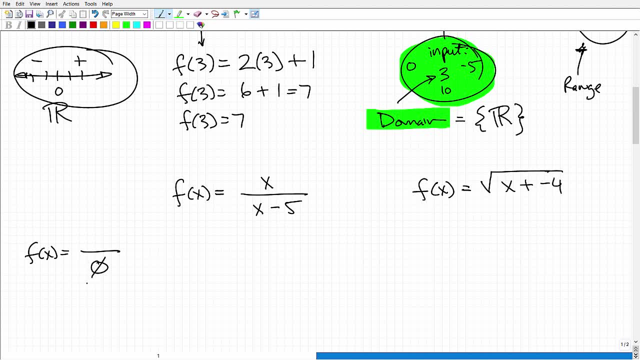 and the denominator. okay, go you. go to your calculator and take 7 divided by 0, not 0 divided by 7, 7 divided by 0. you'll see you'll get an error. okay, so mathematics that's an undefined operation, so we can never end up with. 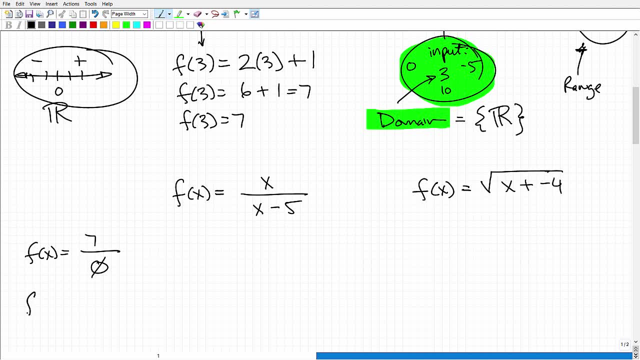 0 and a denominator. that's bad. another thing that we don't want to end up with is taking the square root of a negative number. okay, so in the real number set. that's also not good. okay, our calculators get confused. a square root of a negative number is actually something called a complex number, but 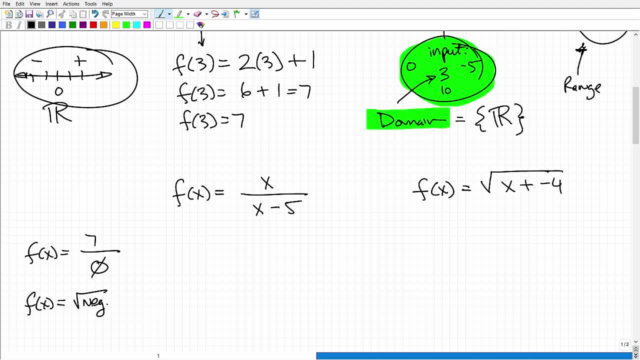 when terms of function restrictions, like again, like what I said, you're gonna be that you're probably in the particular problems they'll say in the set of real numbers. so I'm just telling you, as a math teacher, you know you're gonna have to pay attention. so we don't want a square root, we don't, we're gonna want to. 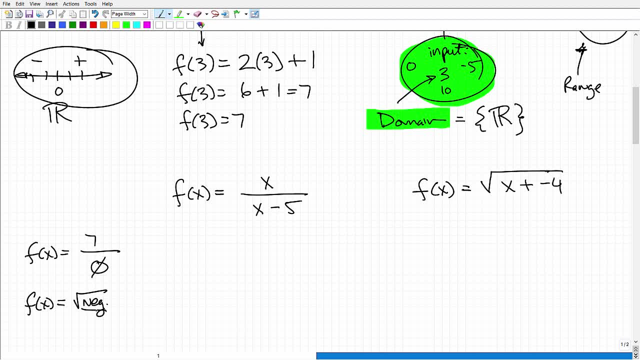 restrict any numbers that cause a negative number value underneath the square root and any values that couple causes 0 to show up in the denominator. so let's take a look at our first example here. so is there any values where such that we plug in something here that will cause a 0 in the denominator? well, clearly there is. 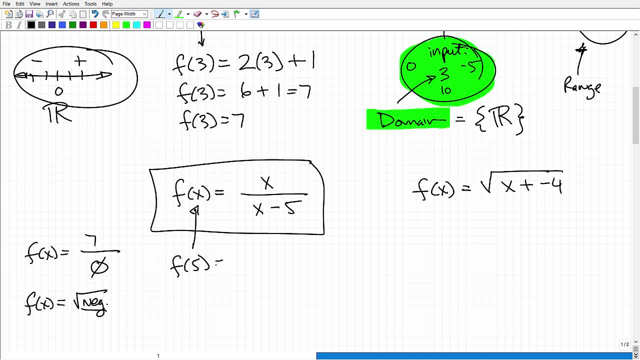 it's 5, right. so if I do f of 5, I'm gonna end up with what? 5 over, 5 minus 5, and 5 minus 5 is going to give me a 0 in my denominator down here, and that's bad, okay. so this 5 is not allowed. so I'm like I. 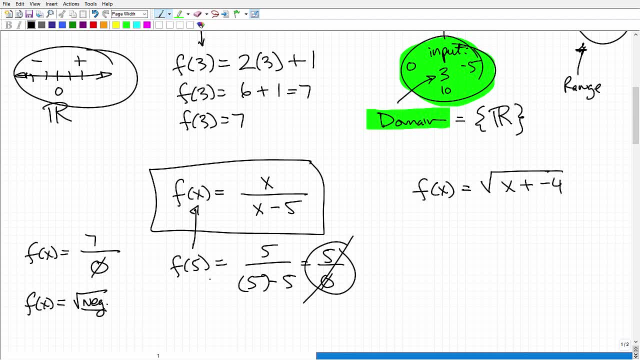 gotta keep you out. 5. you're not. you're not allowed to participate here in the domain. you can't be in the domain team, all right, you can't. you're not gonna be in the set of numbers that are allowed to go into this function, so we got to. 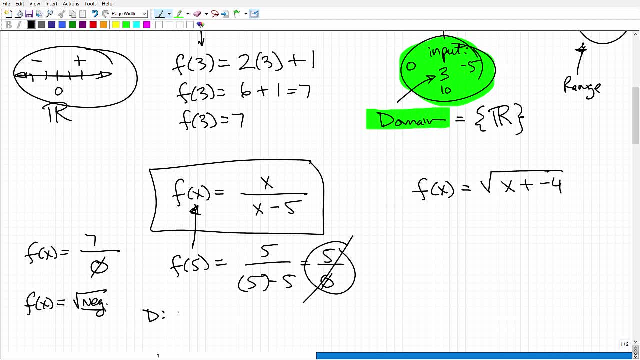 kick it out, okay. so in this case the domain would be: we can write it in all kinds of ways. you could say: it's all real numbers, except X cannot be 5. except x cannot be 5, okay. again, there's various ways to express this, but what i want you to know is that there are. 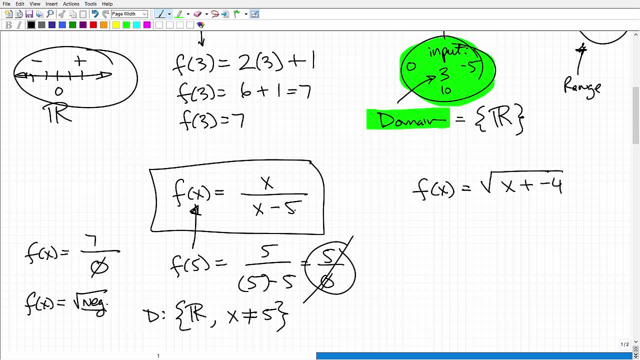 restrictions. so when you see a fraction, you're looking for what value would cause a zero in the denominator. now, by the way, too, you can have a fraction. you can also have, like a negative square roots. this can get much more complicated, but i'm trying to break up these two conditions. 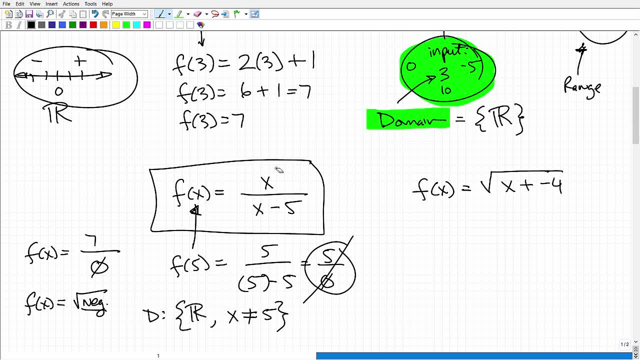 separately. okay, all right. so that's the first condition. now over here i i want to stay away from any x values. that is going to leave me with a negative situation. so, for example, if i'm trying to find what f of 2 is, i'm going to have 2 plus negative 4. i'll end up with the square root of. 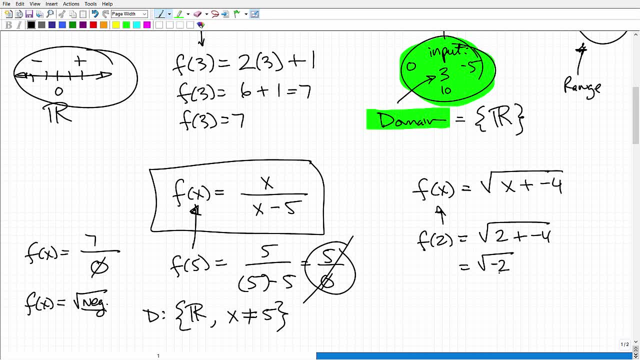 negative 2. that's bad. so when i plug in this 2, i got the square root of negative 2, so 2 is not allowed, but that's only one, one value, okay. so what i have to do in this particular problem is: i got to say: 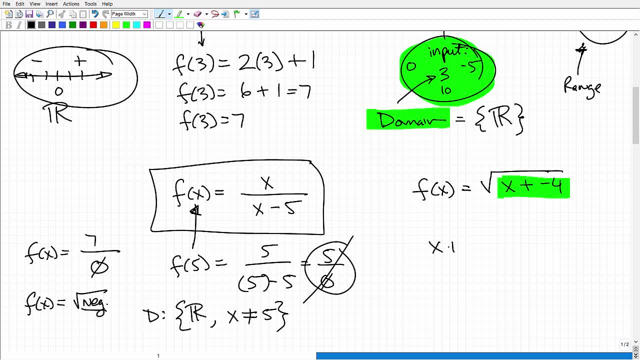 x plus negative 4. okay, i need this to be always what positive or zero. so how can i solve this? well, we can use or how can i um find those values? well, i can use an inequality right to solve. so i can say: x plus negative 4 needs to be greater than or equal to zero, which means 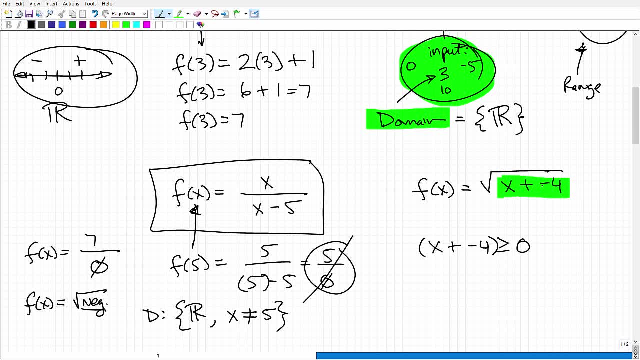 that's positive, right, or 0, 0 is fine, the square root of 0, 0. so when I solve this I'm gonna get X has got to be greater than or equal to 4, okay. so if you think about it, any values less than or so less than 4, like positive 2, is gonna cause a negative. 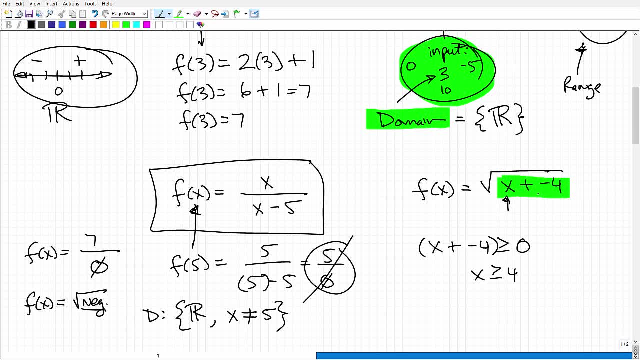 situation: if it's 4, 4 plus negative 4 is 0. that's okay. okay, so in this case, the domain would be real numbers, okay, well, actually we just say it like this: X is greater than or equal to 4. okay, that's fine. all right, because we're talking. 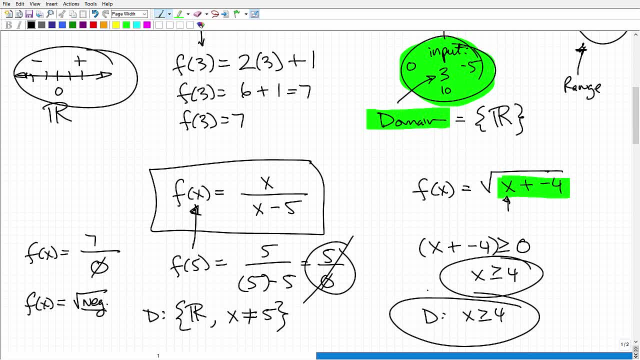 about the real number set. so if you're with me so far and you understand these principles, then that's good, okay, but that does not no way mean that you're like. you know. you need a lot more practice, because there's a lot more. I can make these problems much more sophisticated, much more. 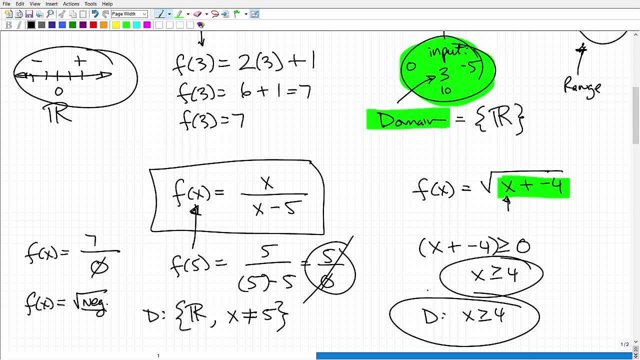 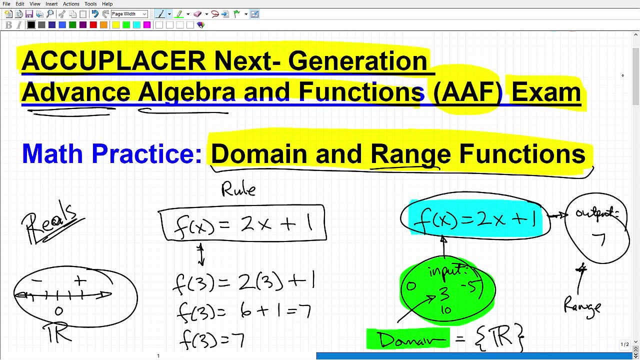 challenging, much more complicated, much more challenging, much more challenging where this factoring involved, etc. etc. but this gives you a sense of the level mathematics that you're going to need to know for the ACCUPLACER, you know, next gen AAF exam. okay, we're advanced algebra and functions right. a little taste of it. 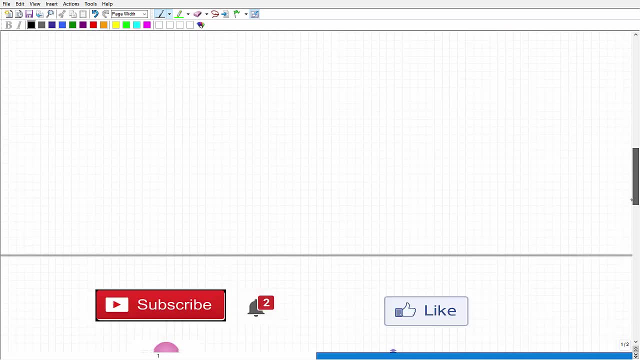 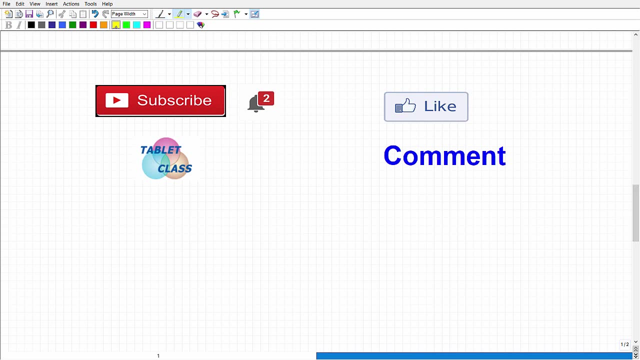 so hopefully you got something out of it. let's go and wrap this up again. you know, my advice to you is to get some sort of good study plan going. use some good study material, trust and study material. you don't have to use any one program. you can kind of use a hybrid if you like my teaching style. again, I have 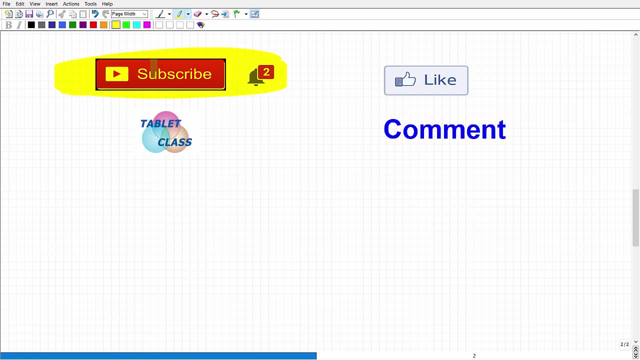 a specific, very comprehensive course specifically for for this exam. the link is in a description of this video. I also have a ton of videos on my youtube channel- literally hundreds- that you can watch, so hopefully you consider subscribing. I'm posting all the time so if you understand the way I teach math, 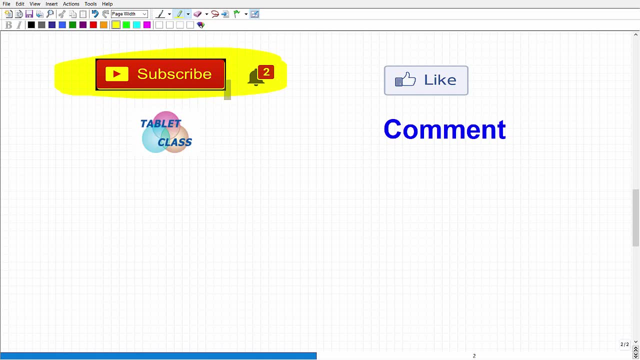 you'd like the way I teach math and then you can get a lot out of my channel, my videos, and you'll get all definitely a lot out of my formal course on this. hey, if you enjoyed the video, definitely appreciate a thumbs up and, last but not least, leave me some feedback. it's the